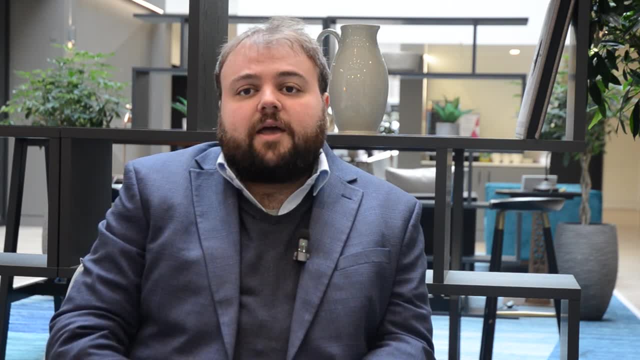 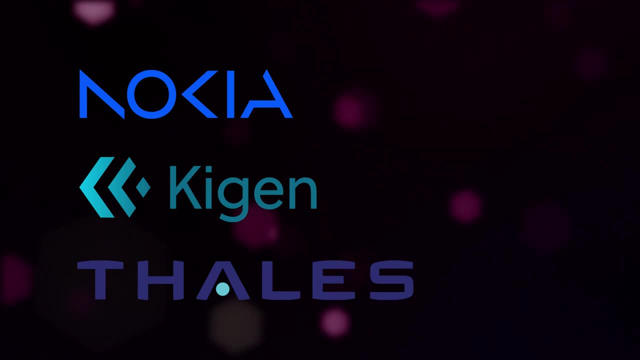 such as identification and security, directly into the software layer of the device in use. During 2023,, we saw a number of launches of iSIM platforms and modules from companies like Nokia, Kaigen and Thales, and in 2024, we anticipate a substantial surge in iSIM adoption. Especially within the IoT space, where the removal of physical SIM modules promises to reduce the device form factors and, in turn, improve devices versatility and energy efficiency. And there is also a clear advantage for vendors. here too, With the complete removal of hardware dedicated to SIM functionality, vendors will enjoy reduced development and manufacturing times. 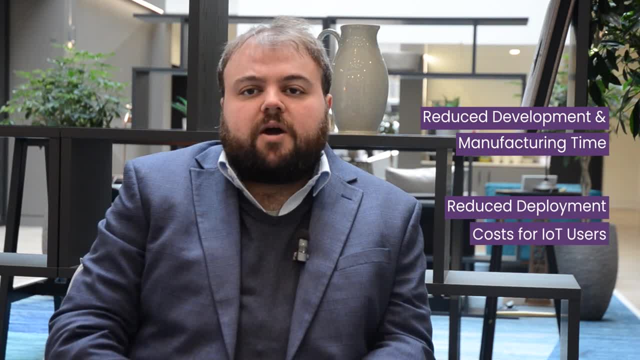 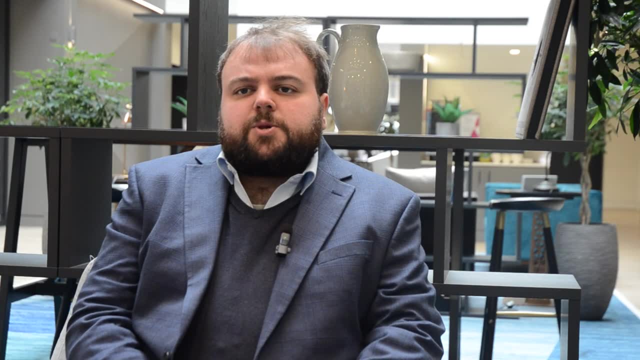 while the ability to use remote SIM provisioning will reduce deployment costs for IoT users. Regardless of your industry, generative AI is a key part of the iSIM industry. Generative AI is a key part of the iSIM industry. Generative AI is a key part of the iSIM industry. 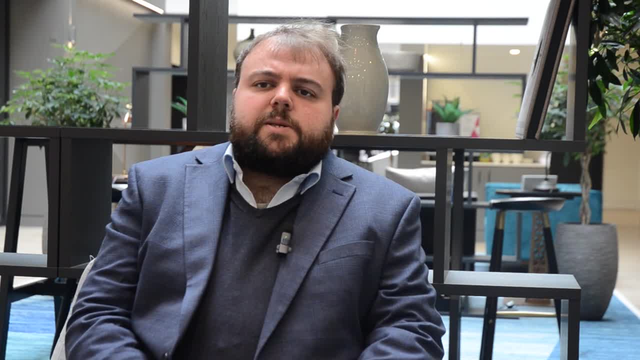 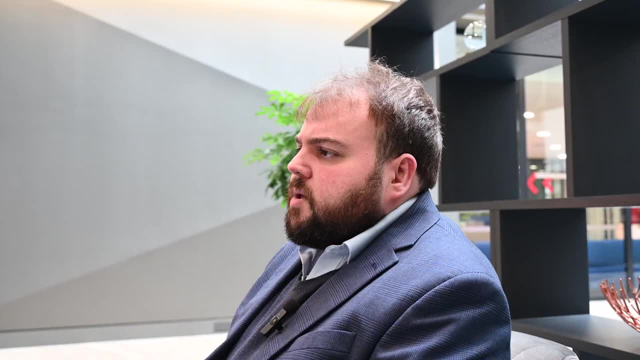 Generative AI was the hottest topic of 2023, and with good reason. By automating the generation of digital content, generative AI has the potential to revolutionize business processes in ways that just weren't possible two years ago. Within the next year, we're going to see CPaaS platforms increasingly embrace the 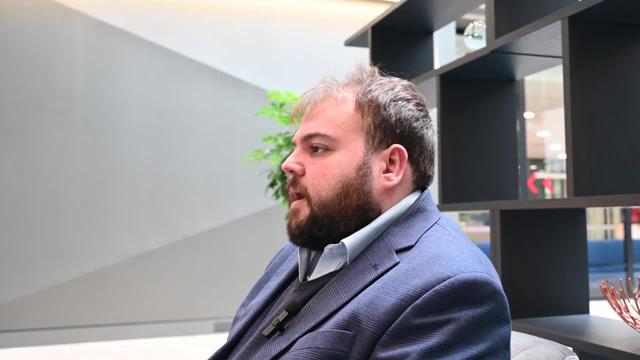 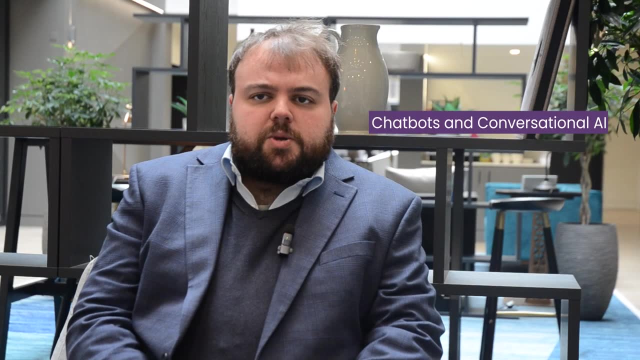 capabilities of generative AI to increase the marketing campaigns over their channels, And there are two major use cases here that we expect to experience traction. Firstly, chatbots and conversational AI. These are chatbots that leverage generative AI and engage with users with personalized conversations. 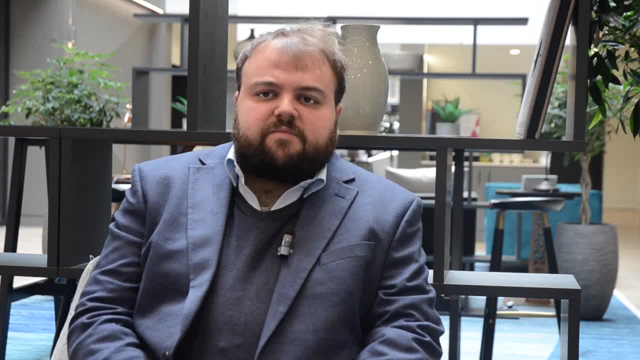 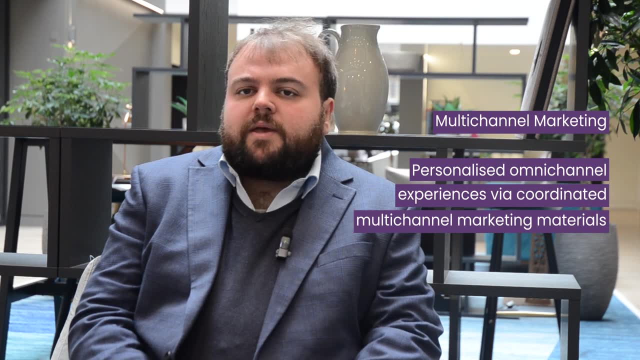 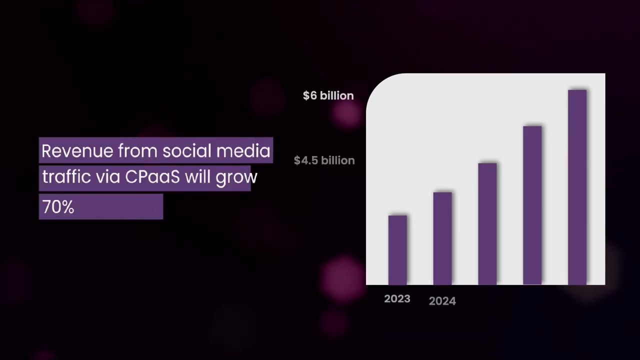 Secondly, there's multi-channel marketing where, through the support of CPaaS and CSPs, enterprises can provide personalized omnichannel experiences through the coordination of marketing materials across various marketing channels to ensure a consistent, tailored experience. Additionally, the growth of generative AI will have a significant impact on the growth of emerging 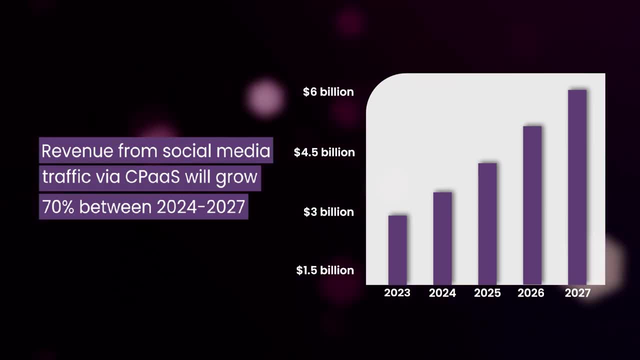 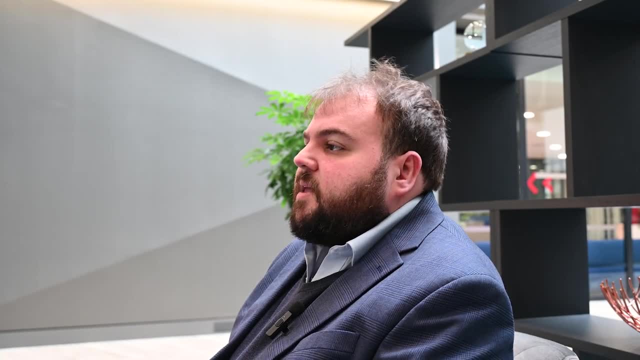 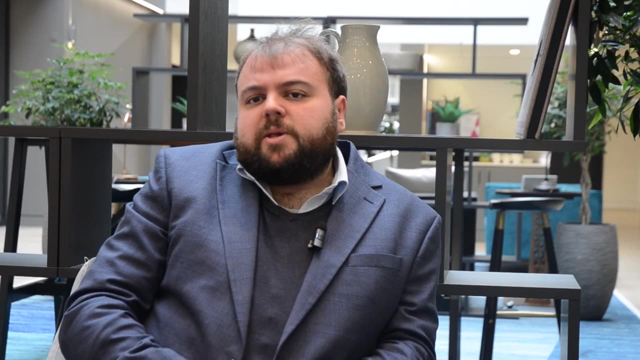 CPaaS channels, most notably social media and the ability to automatically generate personalized content, as well as provide a solid differentiation point to CPaaS vendors looking to distinguish themselves in a collaborative way. And finally, there's the clouding marketplace. While mobile messaging channels are a key part of many enterprises' business strategies, 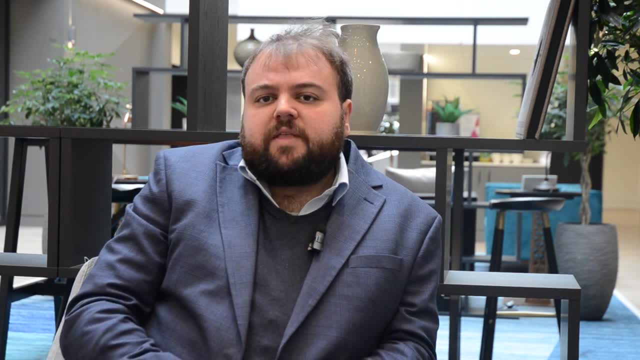 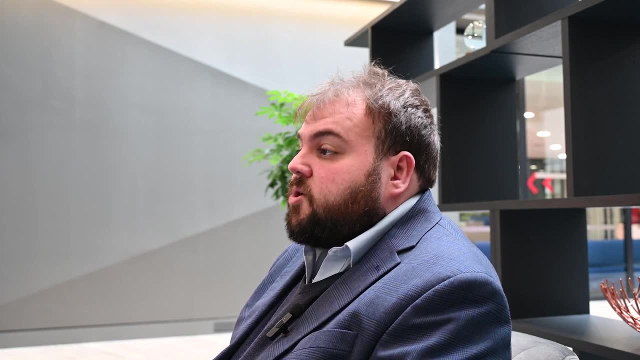 voice will remain a core service for enterprise communications over the next five years. Next year, following on from their successes in 2023,, we expect large language models such as ChatGPT, Microsoft Bing and Google Bard to capitalize on this demand by launching services.